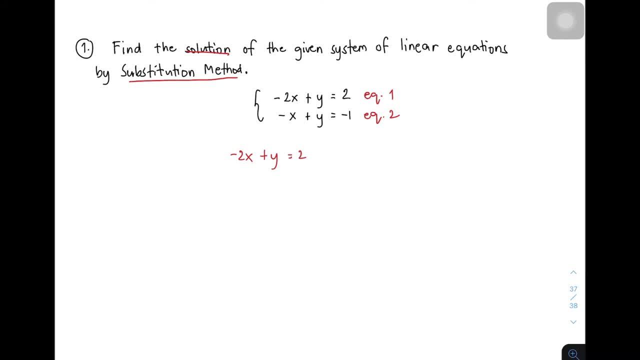 Our target is to solve for Y. okay, solve for Y tire. so we have. transpose negative 2x to the other side of the equation so you can use: Y is equal to 2x plus 2. this will be your third equation, so you have equation number three now. 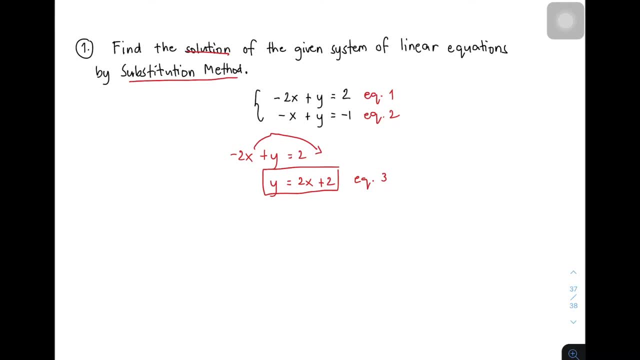 what we will do is use equation number three is for you to substitute this to the other equation that we haven't used yet. basically, we have used equation number one, so we will be using equation number two: negative X plus Y, X plus Y. X plus Y is equal to negative 1. 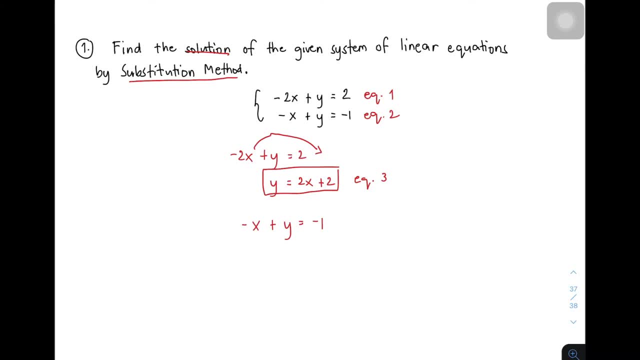 if you notice the equation number three we will focus on, Y is equal to 2x plus 2. the value of Y is equal to 2x plus 2, meaning we can substitute 2x plus 2 to our Y variable, because that is the value of Y. 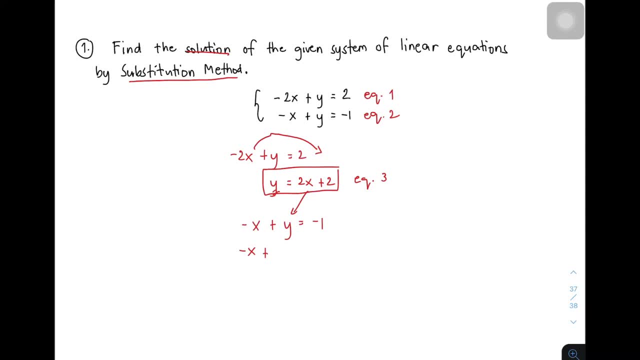 so you have negative X plus the quantity of negative 2x plus 2 became negative 1. so what we need is homebrewing negative X, which can be combined with negative X. that gives you x plus 2 is equal to negative 1, so you can look at it. 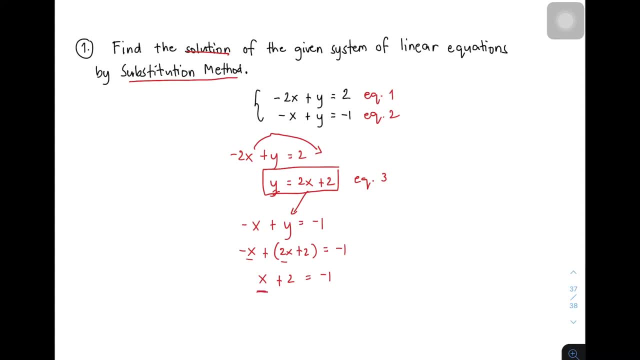 and you can see that there is a variable X right now- shift both to the other side of the equation so we can transpoche to the other side of the equation V. in between we have the variable x, which is negative- 1 minus 2- and then solving for x, it will. 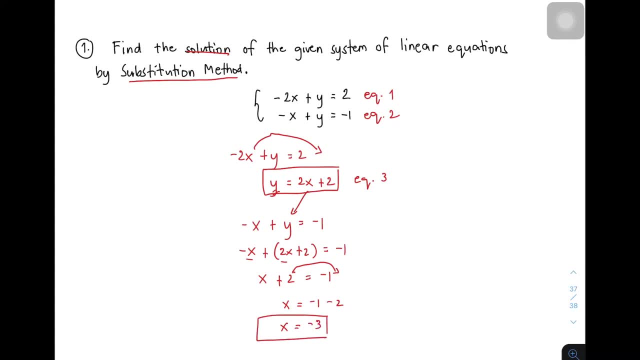 give you negative 3. this is the first value that we got in substitution method. we got the x, so since you already have the variable x, you can solve now for the variable y. sir, which equation will we use? we will be choosing from equation number one or equation number two, so what we can use. 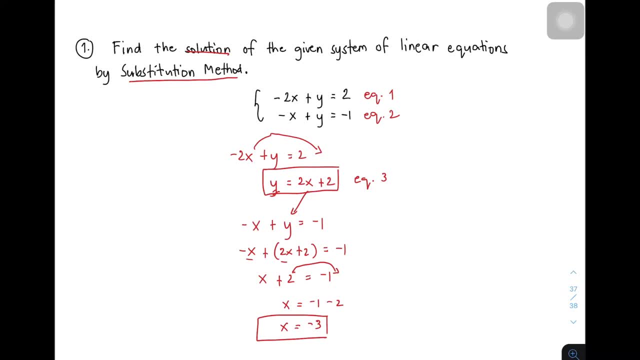 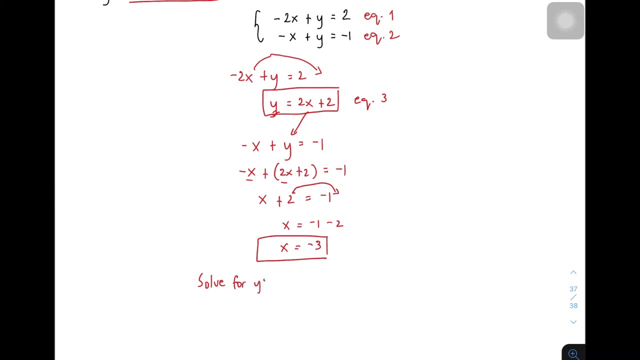 is equation number two. so your equation number two is negative x plus, let's say, solve for y. solve for y because we already have x, so you have negative x plus y is equal to negative one, your x is equal to negative three. let's change that. so what we get here is negative times. 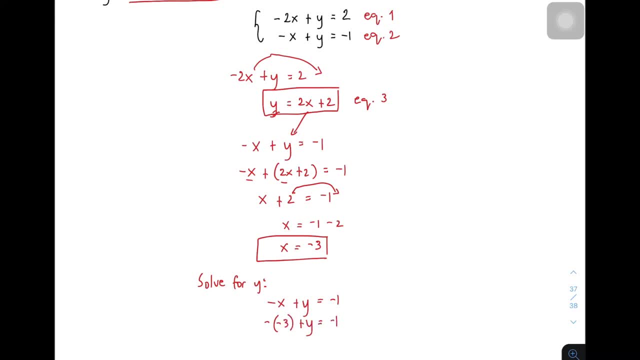 negative. three plus y is equal to negative one. and then solving for this, it will give you negative times, negative, that is positive. three plus y is equal to negative one. transpose the other three, it will give you y is equal to negative, one minus 3. so negative one minus three from positive is 3 and y is also negative. 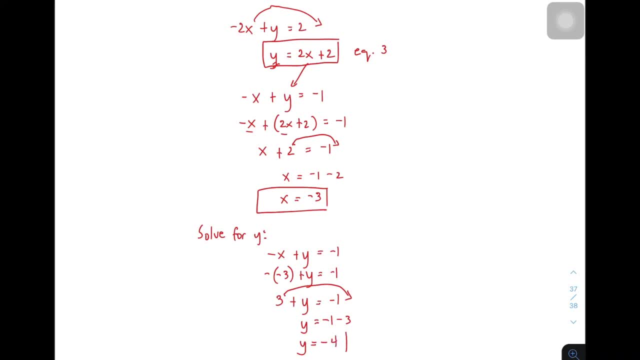 so we get negative 3 because- so you have here- y is equal to negative 4. this is the value of y. so, if you note, we have x and y. in other words, we got the solution already. in other words, the solution of the given solution. industries and eBay. there are three pacts on this screen. so this method brings us to consideration that we need to write a solution now. so if we can just write it, we can just write it and we can have our designsdropped. 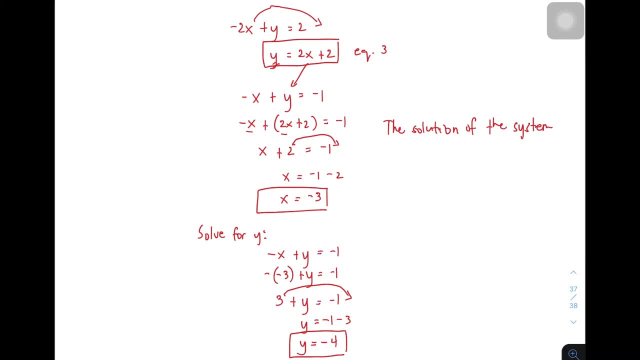 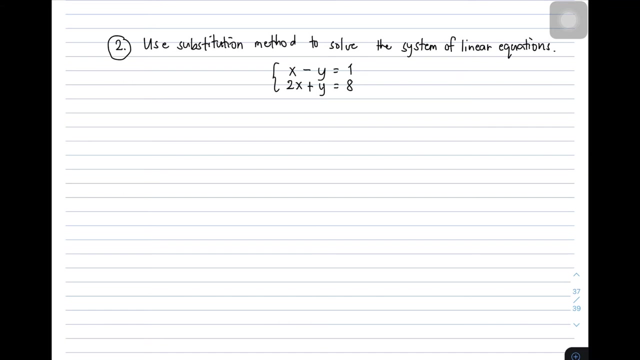 this method is important. use only the teaches. The system of linear equation is negative, 3 comma, negative, 4.. That's it for our first example. So we have here example number 2.. Use substitution method to solve the given system of linear equations. 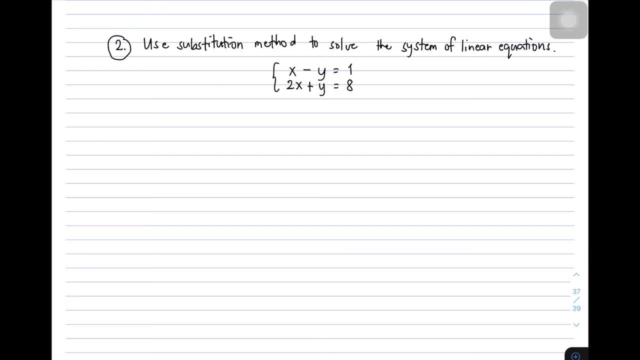 So the given system here is that we have: x minus y is equal to 1. This will serve as your equation number 1.. And then 2x plus y is equal to 8. This will serve as your equation number 2.. 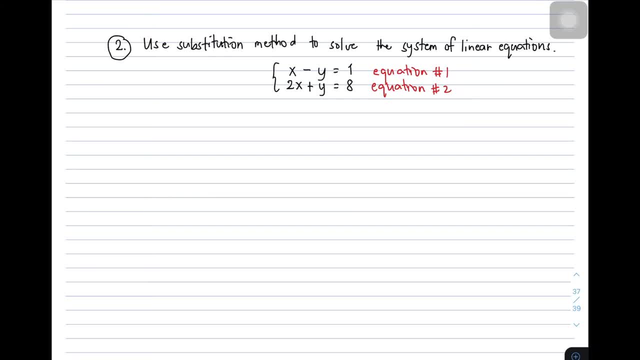 So again, my tip for you is to choose an equation where one of its variables is negative And there is a coefficient of 1. So here we can use equation number 1.. Your equation number 1 can be transformed. Let's write it first. 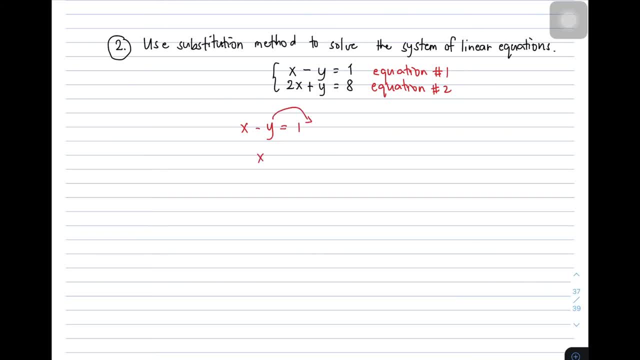 So let's transpose negative y on the other side of the equation. This will give you: x is equal to y plus 1.. So this is the initial value of x. So now, since we have the value of x, we can use this equation to plug in. 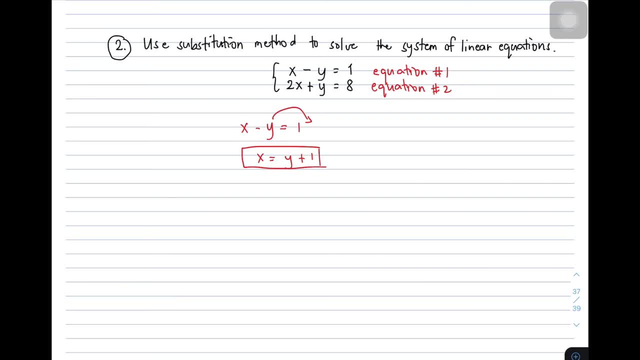 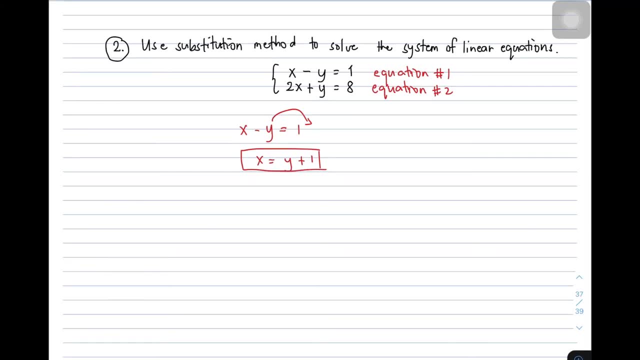 or essentially, we can substitute it in the second equation, since we have already used it. Remember, we have already used equation number 1.. So our next step here is to use the second equation. 2x plus y is equal to 8.. 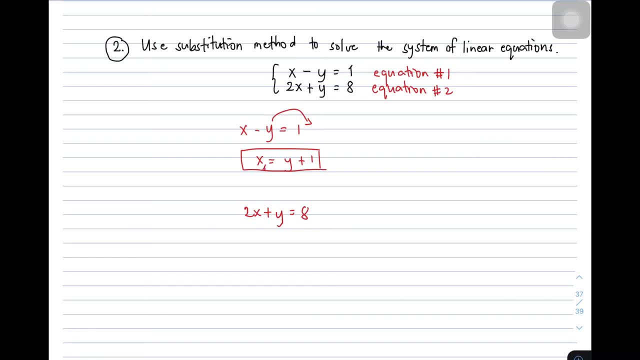 So here in equation number 2, we will plug in the value of x, which is y plus 1.. If we notice, we will plug in the value of x here and substitute it. So let's try it. So you have 2 times. 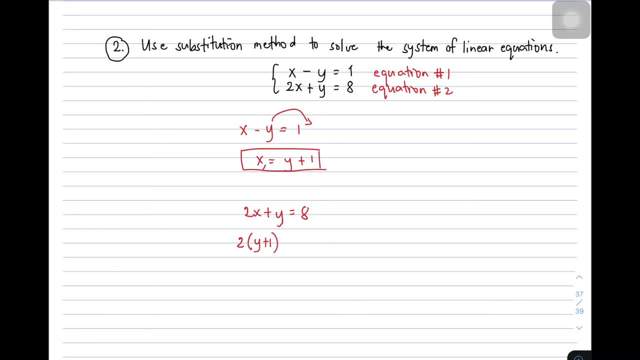 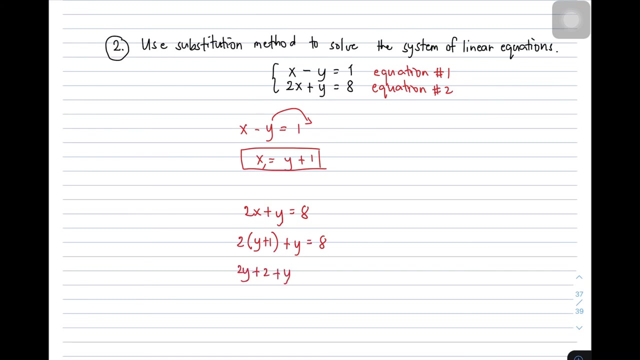 our x will be replaced by y plus 1 plus y is equal to 8.. And simplifying this by distributive property, it will be 2y plus 2 plus y is equal to 8.. And simplifying combining like terms: 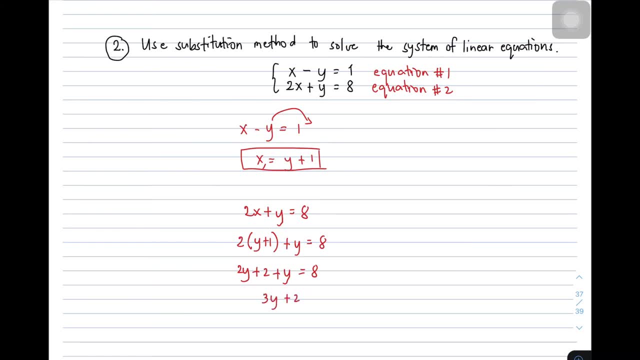 you can have. you can have: 3y plus 2 is equal to 8.. Right after this, let's transpose the 2 on the other side. It will give you 3y is equal to 8 minus 2.. And let's simplify. 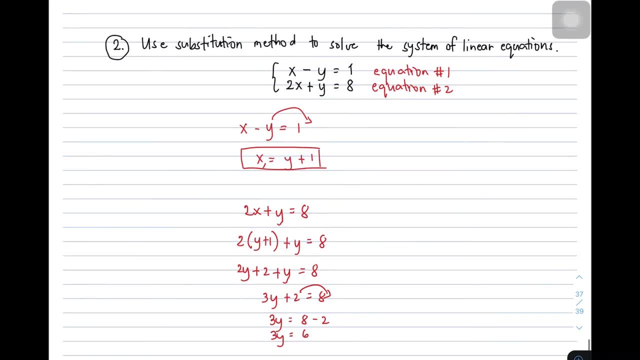 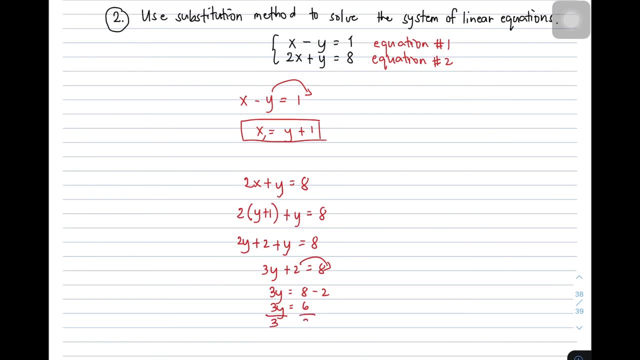 You have, 3y is equal to 6.. Divide both sides by 3.. So the value of y is equal to 2.. This is the value of y, But we're not yet finished. Remember, we're not done yet. 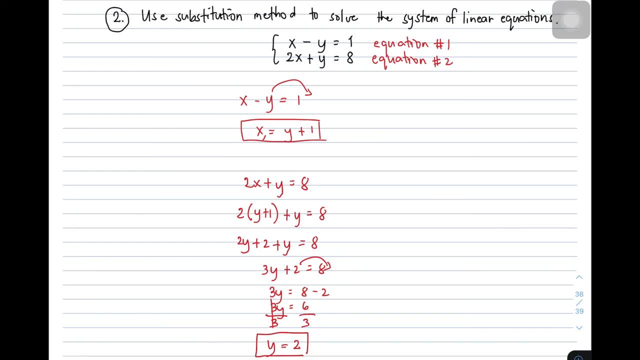 So if we have the variable y, we can still solve for the variable x. So what I'm going to use now is the first equation. You have x minus y. Again, I can solve for y. I solved for x. You have to use x minus y is equal to 1..